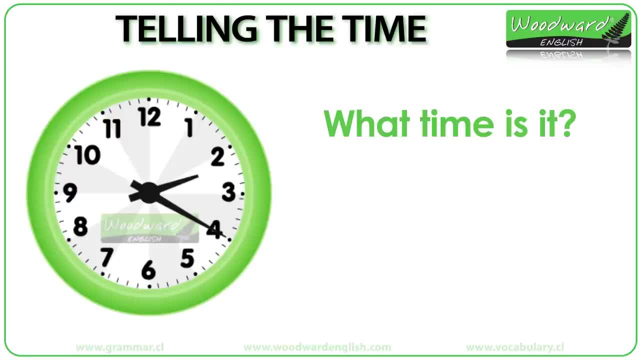 What time is it? It's twenty past two. What time is it? It's twenty five past two? What time is it? It's half past two or it's two thirty? What time is it? It's twenty five to three. 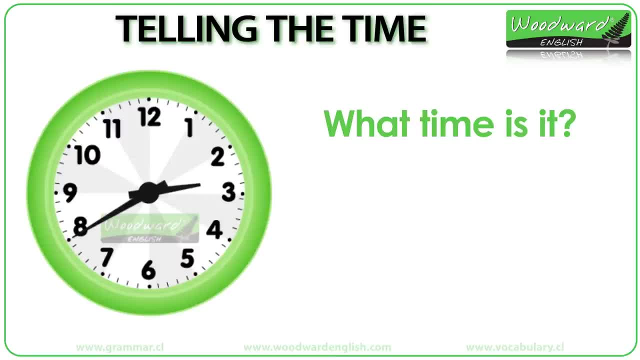 What time is it? It's twenty to three. It's twenty to three. What time is it? It's quarter to three. It's quarter to three. It's quarter to three. What time is it? What time is it? It's ten to three. 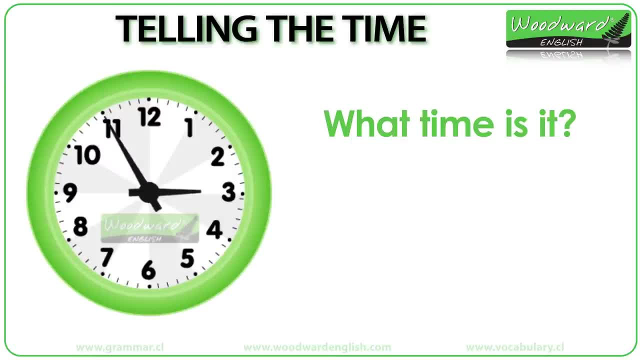 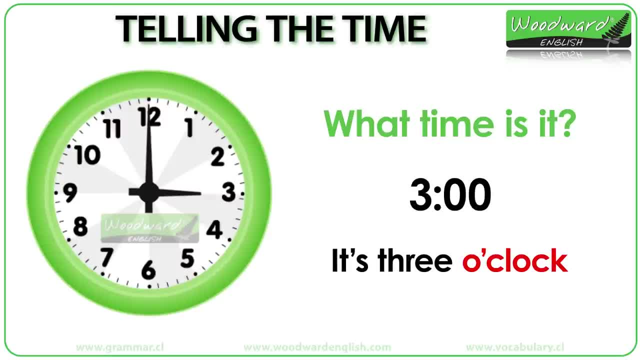 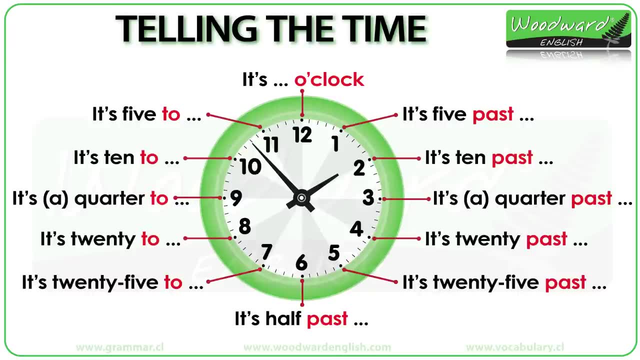 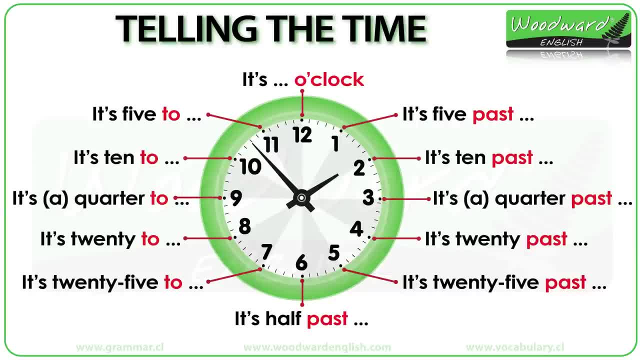 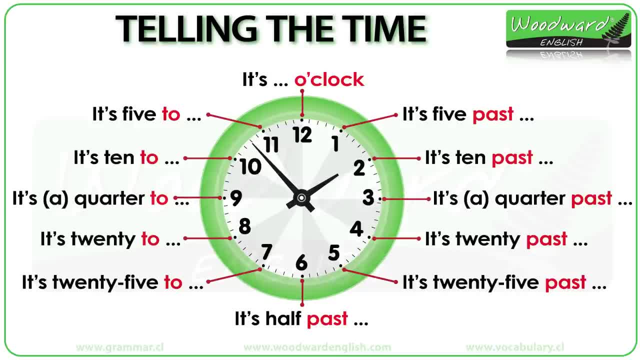 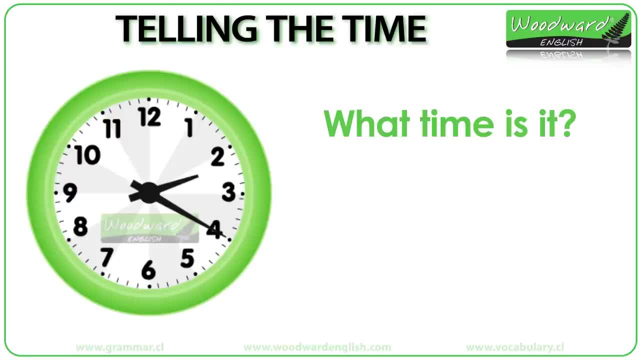 What time is it? It's twenty past two. What time is it? It's twenty-five past two. What time is it? It's half past two or it's two-thirty. What time is it? It's twenty-five to three. 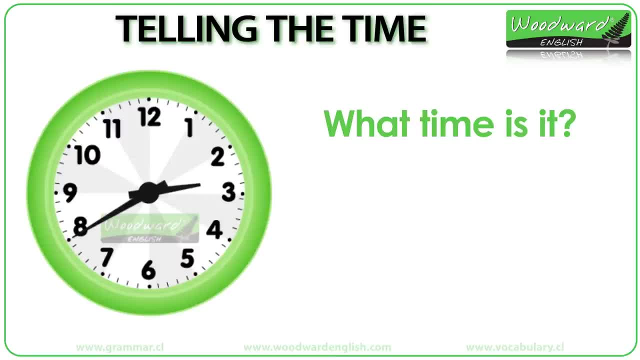 What time is it? It's twenty to three. It's twenty to three. What time is it? It's quarter to three. It's quarter to three. It's quarter to three. What time is it? What time is it? It's ten to three. 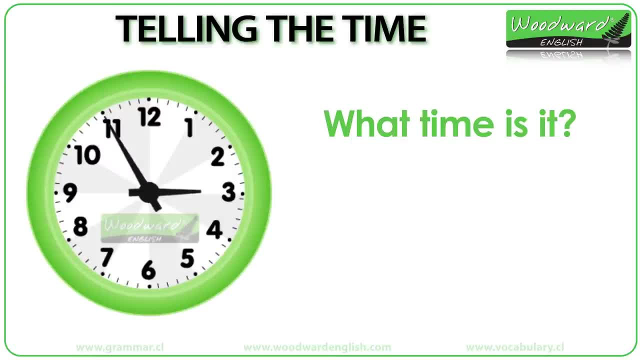 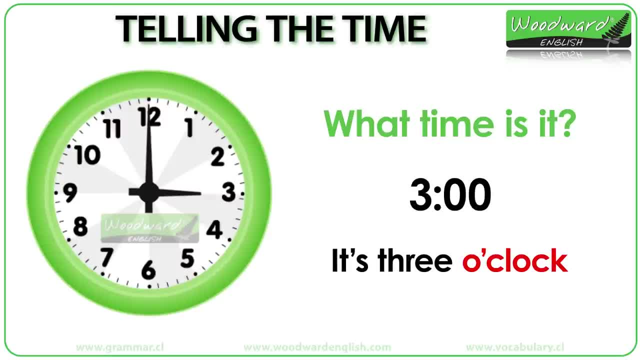 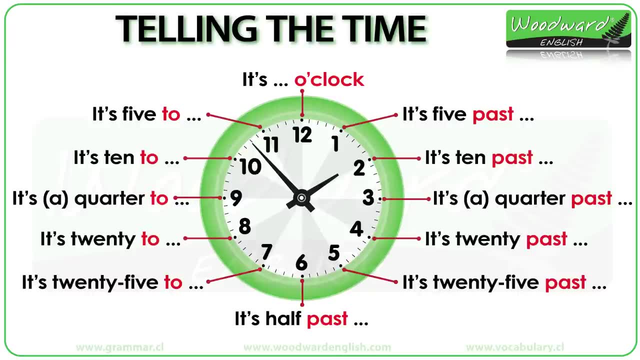 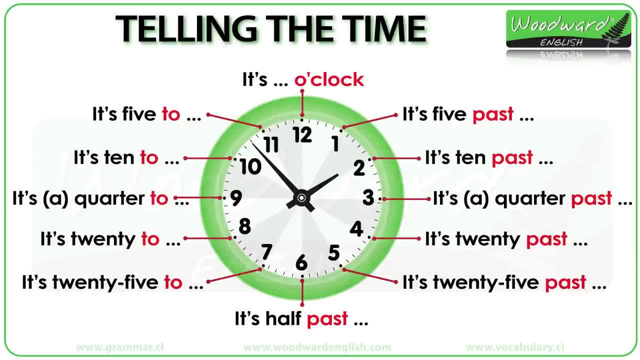